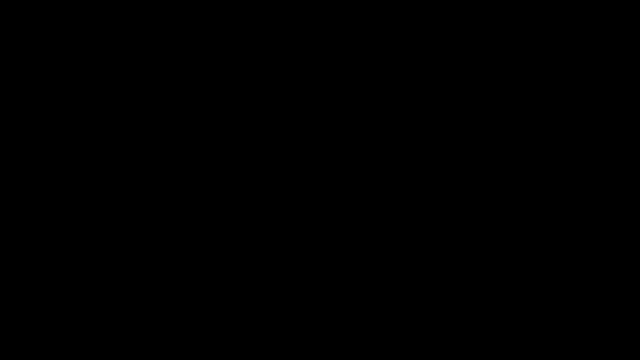 So in this tutorial, we're going to focus on hydrogen bonding. So when you hear the words hydrogen bond, what do you think about? What is a hydrogen bond? A hydrogen bond is a dipole-dipole interaction. In fact, it's a very special type of dipole-dipole. 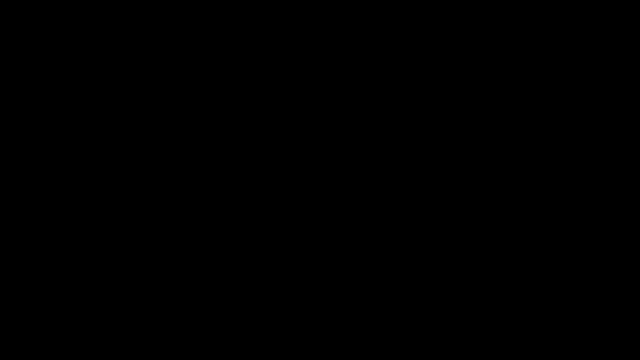 interaction. It's a very strong type of dipole-dipole attraction force. Hydrogen bonds occur whenever hydrogen is directly attached to nitrogen oxygen or fluorine. Let's compare the HF bond with the carbon-oxygen bond. Both of these bonds are highly polar. 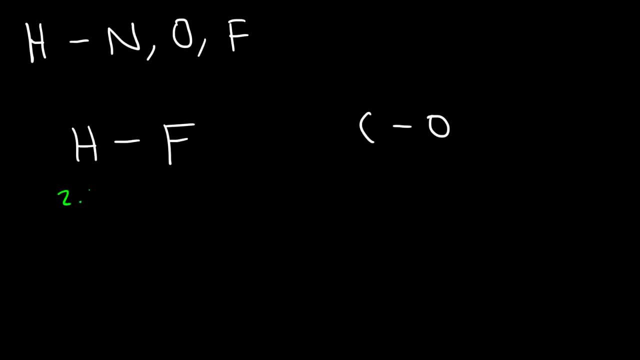 The electronegativity value of hydrogen is 2.1 and of fluorine is 4.0.. For carbon it's 2.5 and for oxygen it's 3.5.. So, for example, the carbon monoxide molecule is a polar molecule. It has dipole-dipole. interactions. Now, HF is also polar, but it has a special type of dipole-dipole interactions known as hydrogen bonds. So why are hydrogen bonds a lot stronger than dipole-dipole forces, even though they work the same way? Well, for one reason. the HF bond is more polarized than the CO bond: The electronegativity. difference is a lot bigger in HF It's 1.9 compared to 1.0 in CO. So hydrogen bonds are highly polarized. That's one reason, And the second is that hydrogen is a very small atom. Hydrogen is very small compared to carbon. The average atomic radius of hydrogen is 37 picometers and for carbon it's 77 picometers. So those are the two reasons why hydrogen bonds are a lot stronger than dipole-dipole interactions. It's because those bonds are highly polarized. There's a huge electronegativity difference. 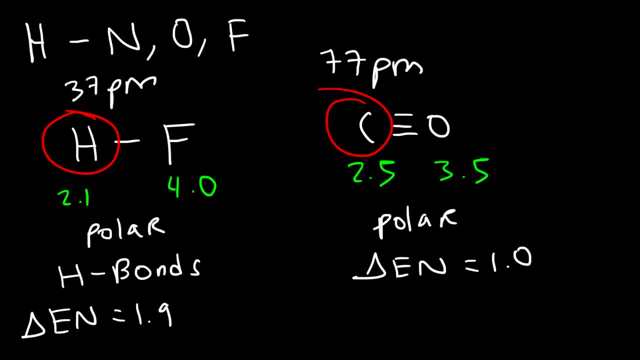 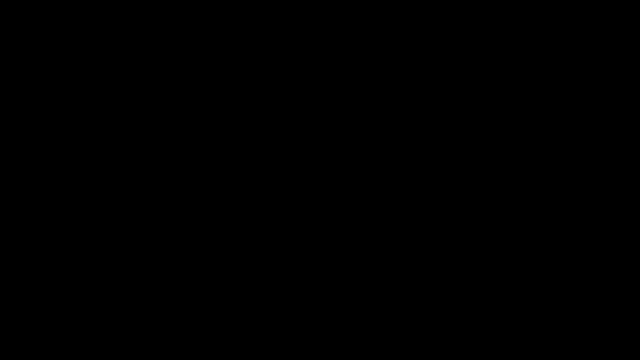 and also because the atoms involved are very, very small. Now to illustrate the effect of size on forces of attraction, let's say if we have a positive charge and a negative charge separated by a distance of, let's say, one centimeter, And let's say that the force of attraction that these two fill, we're going to call it F. 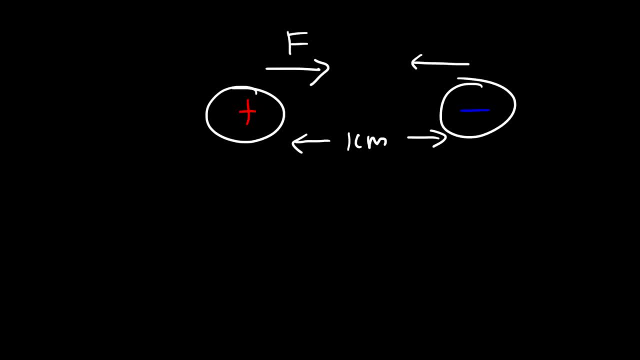 What happens if we have a force of attraction that is equal to the force of attraction that these two fill? What happens if we bring these two charges closer together? So let's say, if we decrease the distance from one centimeter to half a centimeter? 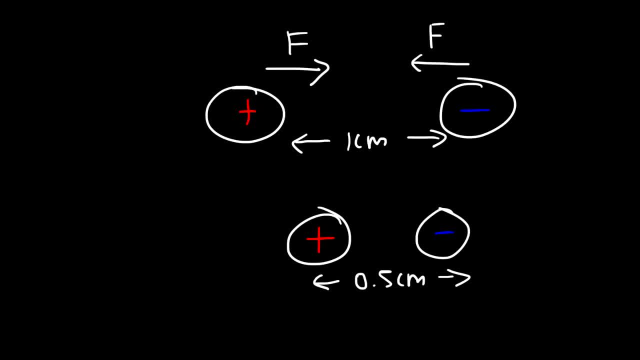 So we reduce the distance by a factor of two. What's going to happen to the electrostatic force of attraction Force is inversely related to the square of the distance. So you can write it like this, if you want: Where R is the distance between the center of the two ions. 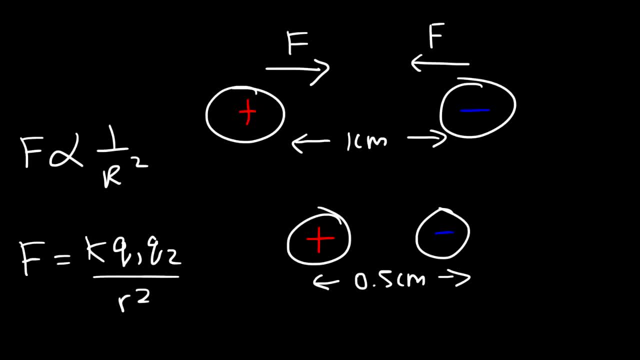 Q1 and Q2 stands for the charges of the ions. So if you decrease the distance between the two charges, the force will greatly increase And notice that it's squared. So one divided by half squared is one over one fourth, which is four. 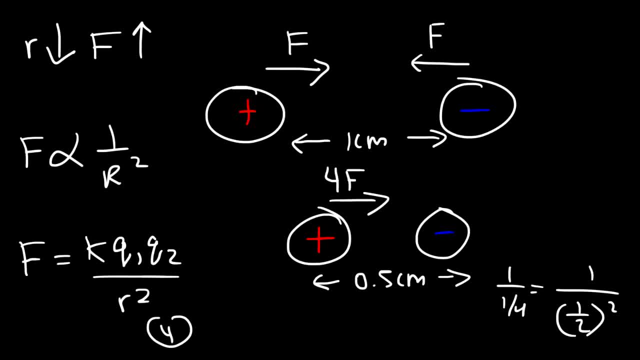 So therefore, the force will increase by a factor of four if you reduce the distance by a half. So because hydrogen is so small, the distance between the nuclei will be reduced, And so the forces of attraction between HF molecules will be a lot stronger than the. 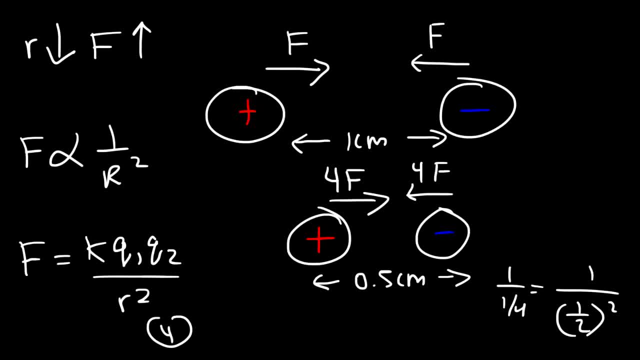 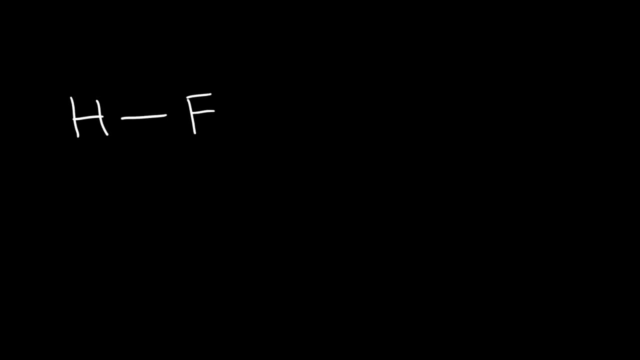 forces of attraction between CO molecules, And so that's why size is important when dealing with electrostatic forces of attraction. If you decrease the size of an electron, the force will increase As we go into theまだ representative molecule. we are dealing with hydrogen bonds. 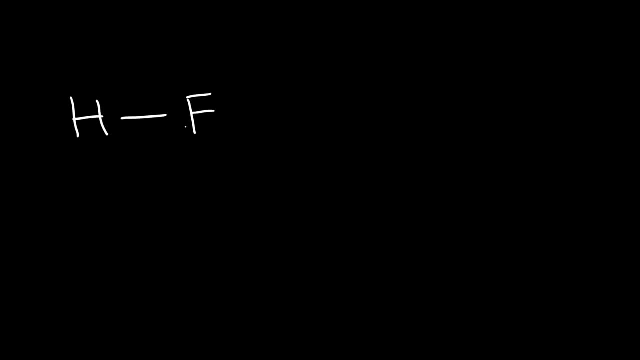 If you want, you can increase the trend and look for these HF molecules close to each other In the selected molecule whose Soviet Russians just worked on. who are these? HFC? alive, Minus the basis of contact between HF molecules. Now let's look at the HF molecules, where the hydrogen bond to exist among the HF molecules is the HF. 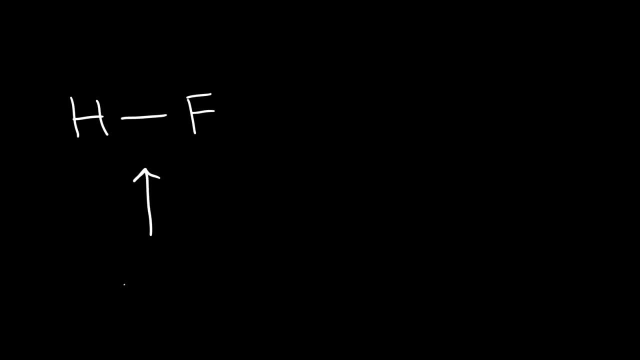 molecule. We want to see the HF current impact, So let's use the HF HF molecule here in the interest freeised cycle to destroy the hydrogen bond. It's equal to the strength that has the HF molecule, meaningless to the significant force of attraction. 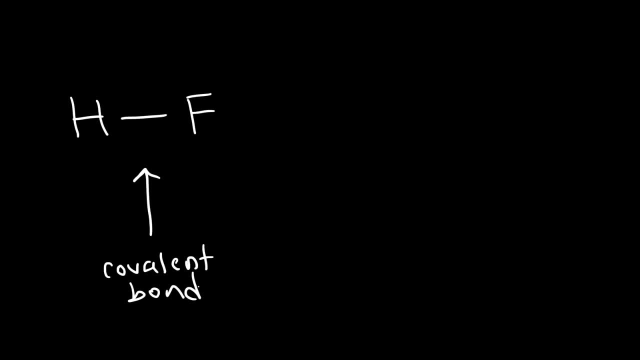 So we want to find two different levels of attraction in onechair so we could use it to measure Earth's current and weight of the electron of attraction that brings the hydrogen and fluorine atoms together. The hydrogen bond exists between molecules. It's an intermolecular force. 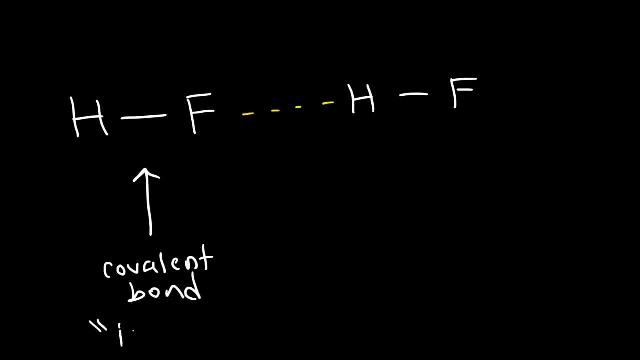 Inter means, between, Intra means, within. So don't confuse an intermolecular bond with an intermolecular hydrogen bond. So that's the H bond. So make sure you understand the difference between an intermolecular force and an intermolecular force. 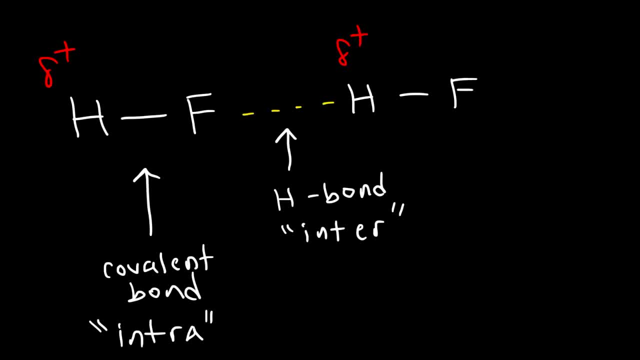 Hydrogen has a partial positive charge And fluorine has a partial negative charge. So the fluorine of one HF molecule is attracted to the hydrogen of another HF molecule And so that force of attraction between HF molecules is the hydrogen bond. So water also has hydrogen bonds. 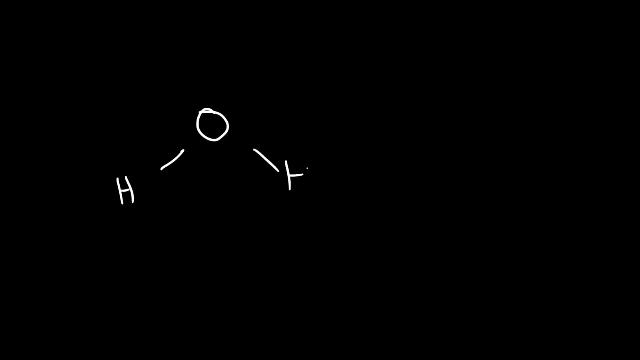 The oxygen atom of water carries a partial negative charge And the hydrogen atoms are partially positive, So water molecules are attracted to each other. So the oxygen of one water molecule is attracted to the hydrogen of another, And so that is the H bond within water. 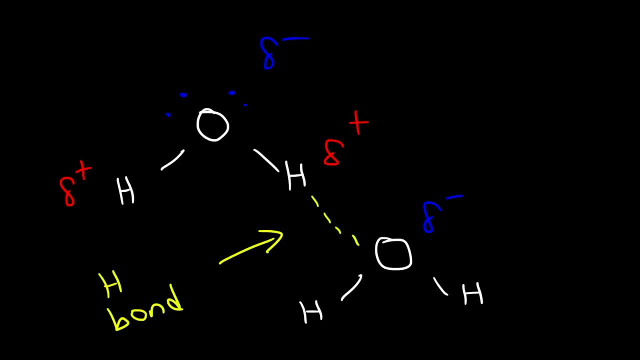 So hopefully this makes sense to you, because it's very important that you understand that. So this is a covalent bond, It's an intermolecular force of attraction, And this is an intermolecular bond or hydrogen bond. So that's the hydrogen bonds that exist between water molecules. 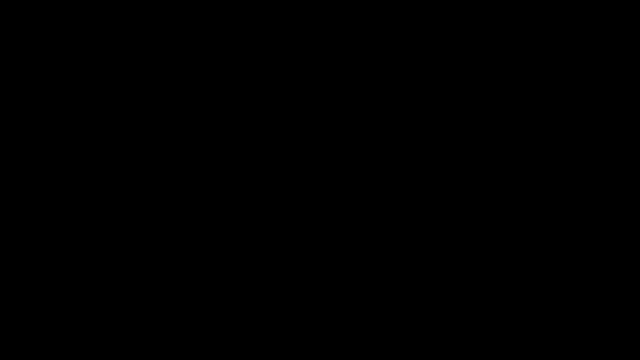 So now, at this point, I want to compare the energy differences between breaking a covalent bond with breaking a covalent bond. So I want to compare the energy differences between breaking a hydrogen bond In order to vaporize liquid water into steam. 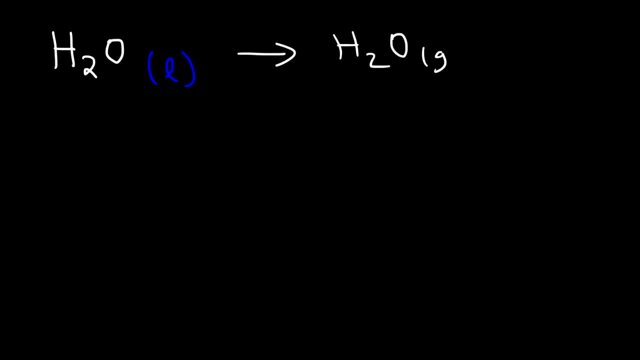 you need to break apart all of the hydrogen bonds that hold the water molecules together. So in liquid water the molecules are relatively close to each other because the hydrogen bonds keep them connected. So in order to vaporize liquid water into steam, you need to break apart all of these bonds and keep in mind to break a bond. 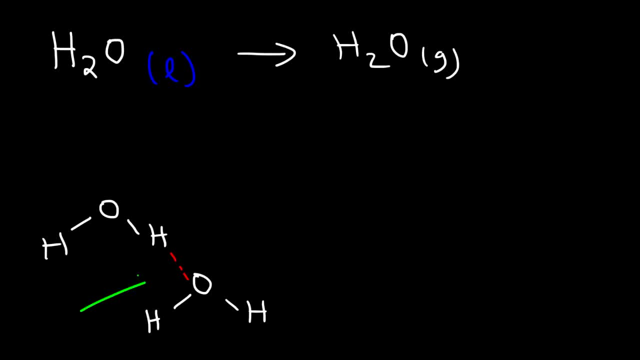 it's an endothermic process. you have to put heat energy into liquid water to break the hydrogen bonds. and once you break the hydrogen bonds, the liquid water molecules will be far apart from each other, in which case they will be in the gas phase. so that's when you have steam. likewise when gaseous steam. 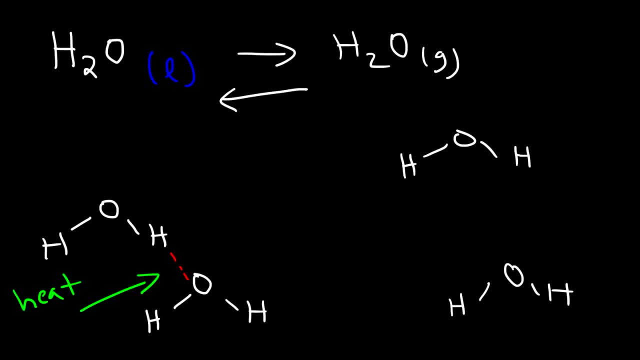 condenses back into liquid water molecules. it regenerates this bond by releasing heat energy. so anytime a bond is formed, it's an exothermic process. heat is released. but to break a bond, it's an endothermic process. that's why if you want to boil liquid water into steam, you got to put it on a stove. you. 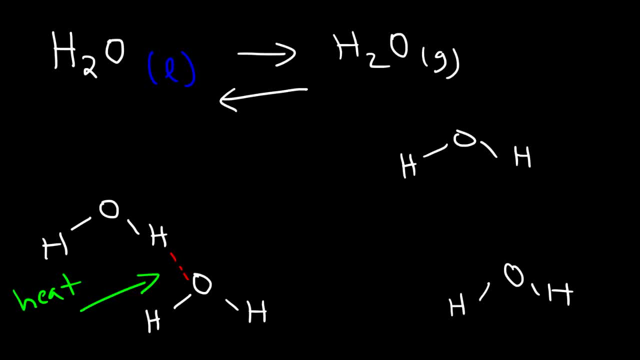 have to add heat energy to it, whereas whenever steam condenses, heat energy is released. so how much steam condenses, heat energy is released. so how much heat energy is needed to break one mole of all of the hydrogen bonds in order to vaporize liquid water into steam? so this is known as the enthalpy of vaporization. 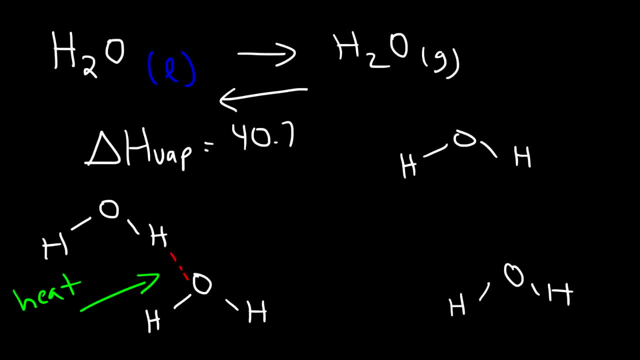 and it's about forty point seven kilojoules per mole. so if you have one mole of liquid water, let's say at a hundred degrees Celsius, you need to add forty point seven kilojoules of thermal energy in order to break all of the hydrogen bonds, so that all of the liquid water molecules could. 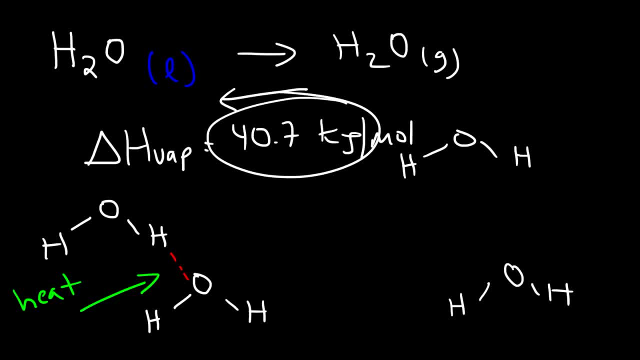 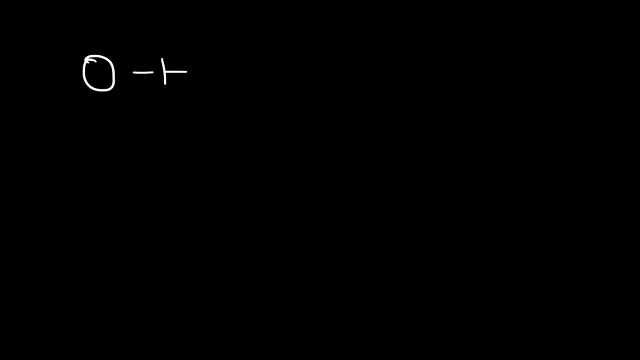 vaporize into steam. so that gives you a good idea of how much energy is required to break a hydrogen bond in order for it to be vaporized into the gaseous phase. now what about a covalent bond? the average bond association energy of an OH bond is: 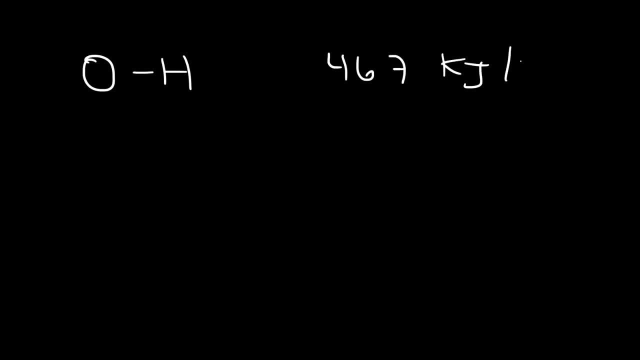 467 kilojoules per mole. so if you want to break one mole of the OH covalent bond, you need to add 467 kilojoules of heat energy. Now, water has two oxygen-hydrogen bonds, and so if you want to break up all of the covalent bonds, 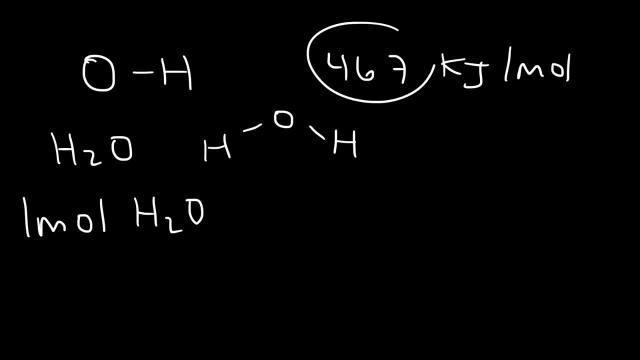 that's found in one mole of water. it's going to be 467 times 2, which is 934 kilojoules of thermal energy. So let's compare that to the enthalpy of vaporization, which is about 40.7. 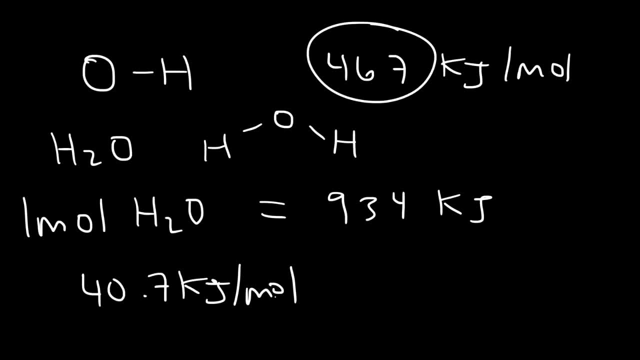 kilojoules per one mole of water. If we divide these two numbers, let's divide 934 by 40.7.. This is about, if you round it to the nearest whole number, 23.. So the covalent bond. 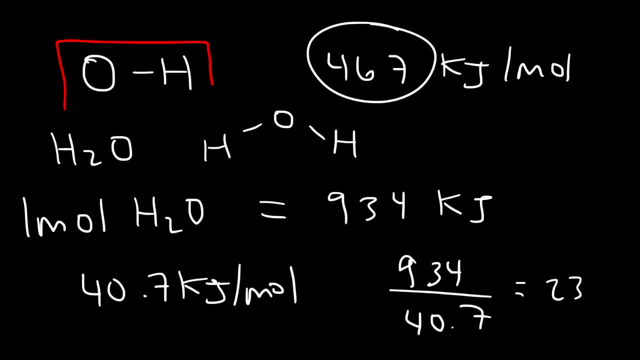 that is, the OH bond is about 23 times stronger compared to the hydrogen bond between water molecules. So, as you can see, a covalent bond is a lot harder to break than a typical hydrogen bond. So intermolecular forces are a lot stronger than intermolecular forces. So the covalent bond is a lot harder to break than the hydrogen bond between water molecules. So intermolecular forces are a lot harder to break than the hydrogen bond between water molecules.